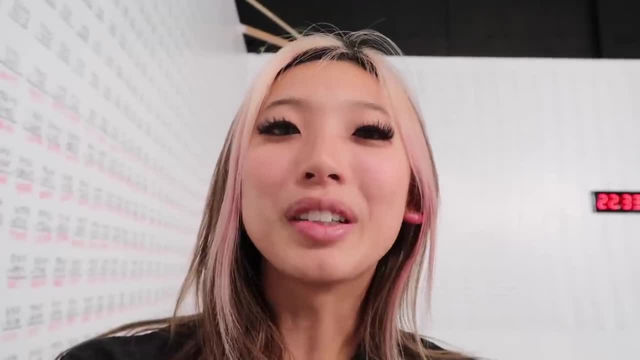 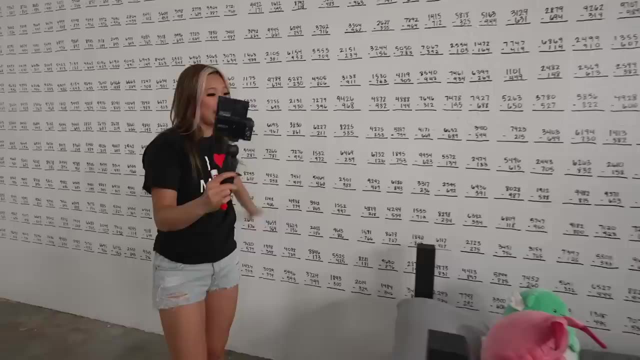 I feel like nobody's gonna recognize me in the thumbnails anymore if my hair changes to blue. I still have multiplication to do. This whole wall is subtraction. I'm not very good at subtraction. I have this cute little bed full of Zach's plushies. 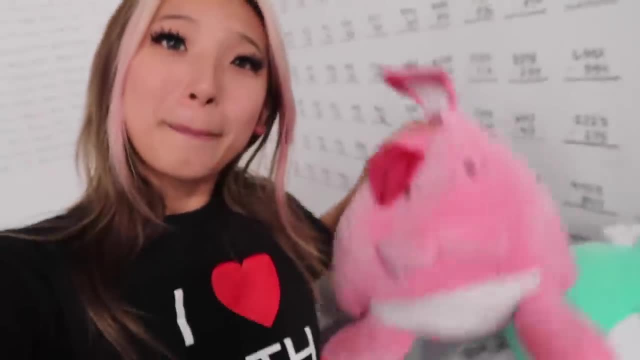 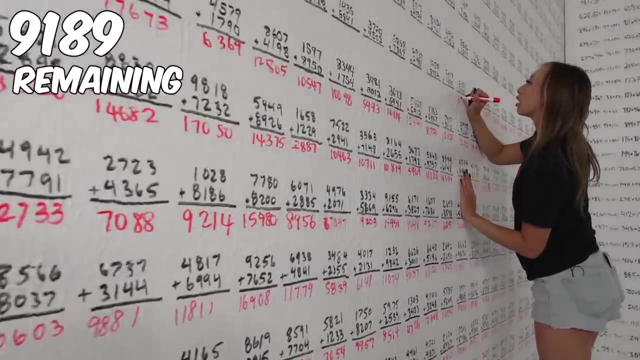 Go to zhdstorecom and buy yourself a cute little bun bun. This bed is for me to sleep on tonight. This is gonna be a really hard 24 hours. Okay, so I've got to the point where I can't reach it anymore. 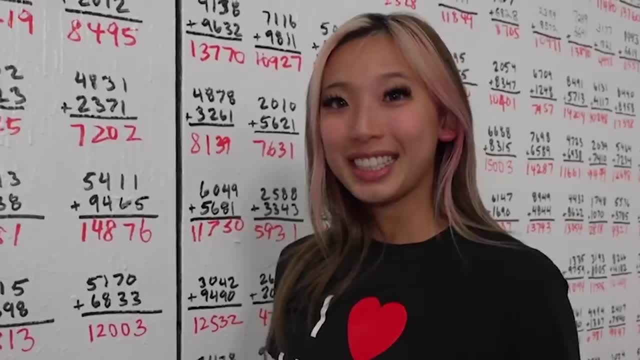 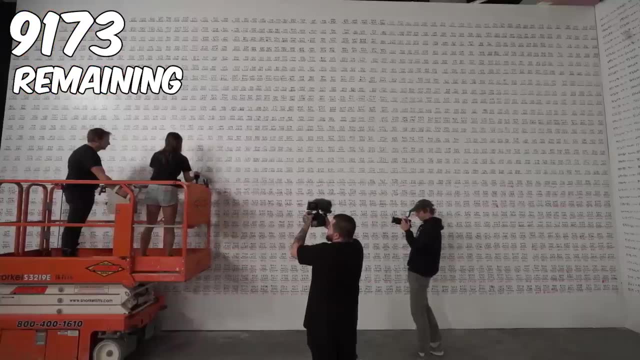 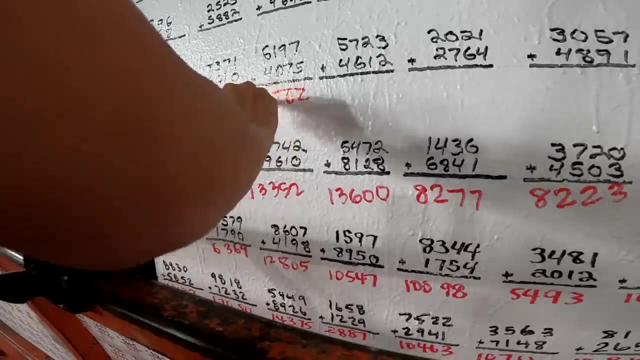 so I'm gonna start using a scissor lift. Scissor lift time Transition. I'm on the scissor lift 826,, 827,, 828,, 829, 830.. Wait a minute, I messed up, It's 10272.. 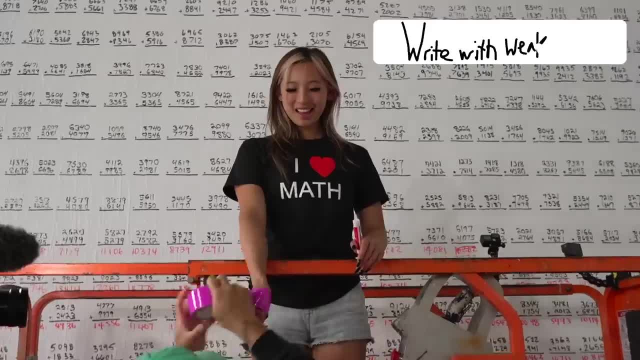 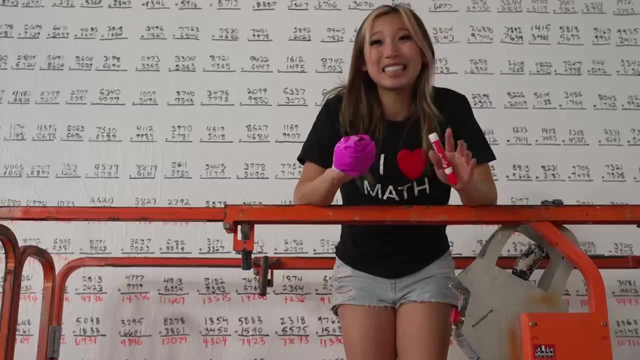 What's the punishment now? Can you tell me? right with you, we can for 10 minutes. No, Yeah, I don't know how to write with my left hand. I've only gone two wrong in the last 900 problems. That's like a 99.78%. 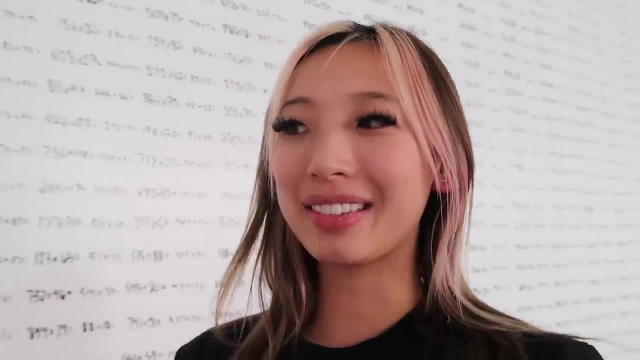 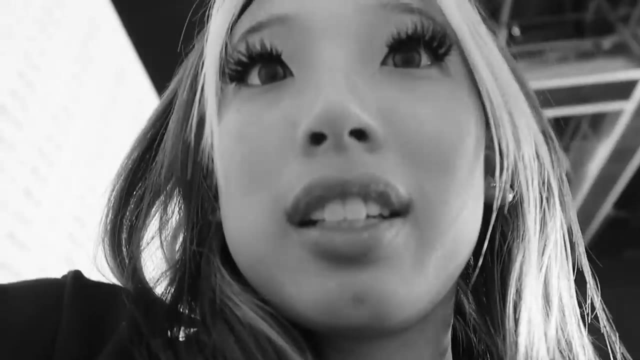 I can't go as fast as I was going before. Writing with my left hand is actually kind of hard. I'm also holding the camera angle really weirdly. If I have to compare this to the world's longest math problem, I'd say this one's a little bit harder. 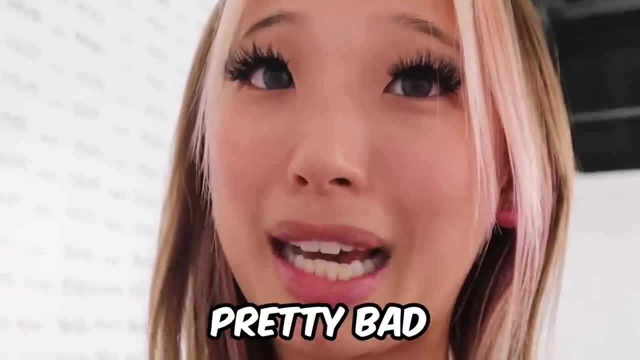 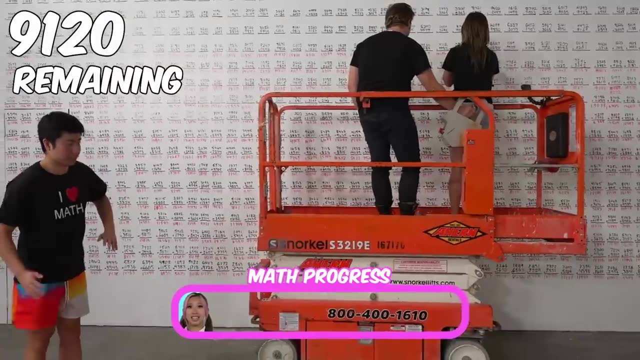 I'm stressing out a lot. The final punishment is pretty bad. Ah Ah Ah, Knuckle hair. I actually have an idea that's going to help raise the stakes. I have a proposal, Not the proposal you've been asking for. 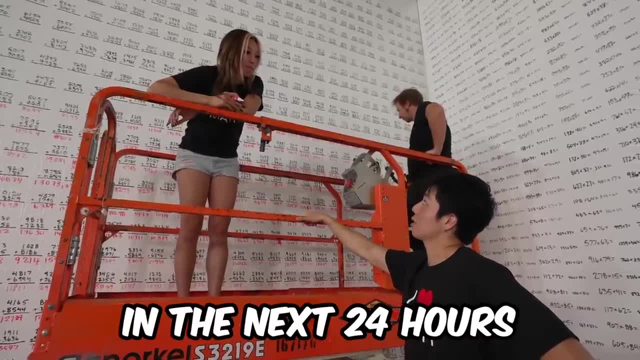 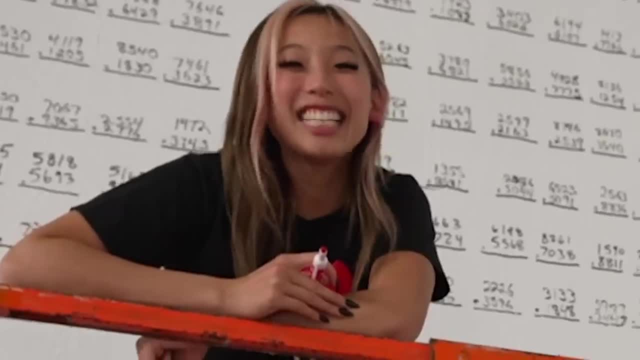 I will give you a dollar for every problem you solve in the next 24 hours. So if you finish all 10,000, I will donate 10 grand to a charity of your choice. I want to donate to a math school Education. 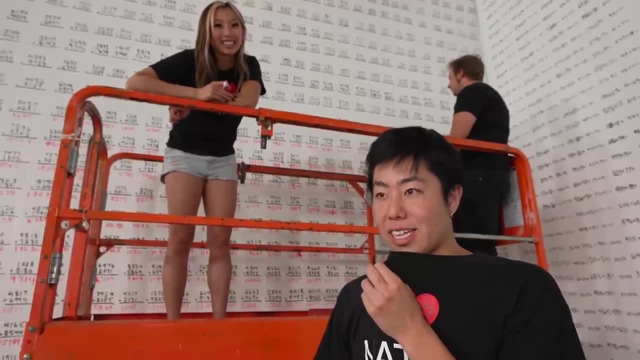 I did hear if you comment, Michelle might take a look at your math class. I don't heart math. I heart Debbie. Comment down below: I love Debbie. Whoa, whoa, whoa, whoa, whoa, whoa. 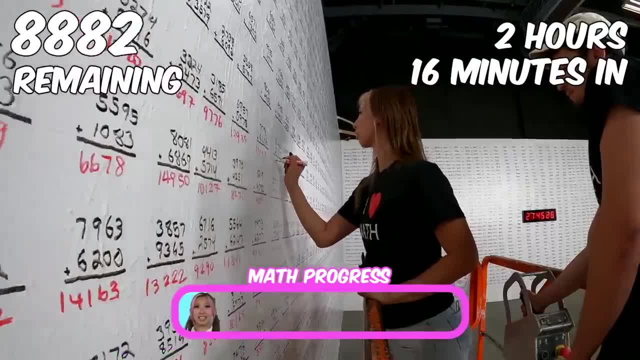 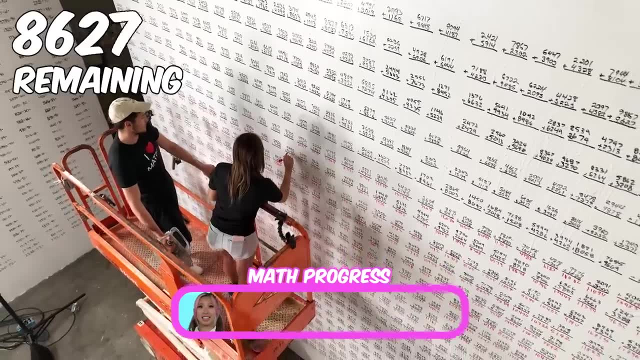 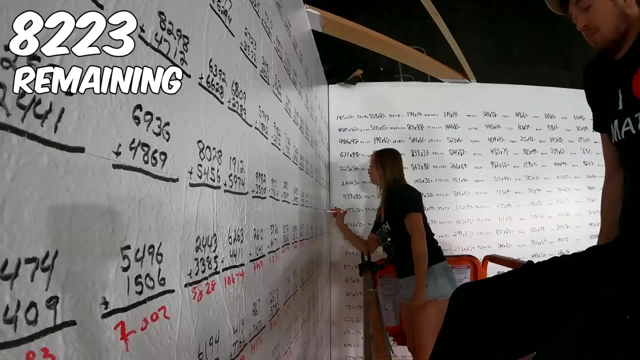 This is much easier than walking. Legs, Legs, Legs. I'm really tired. I still have three other ones left. At this rate, I have to go for 20 hours straight to finish. All right, so I'm gonna mess with Michelle a little bit. 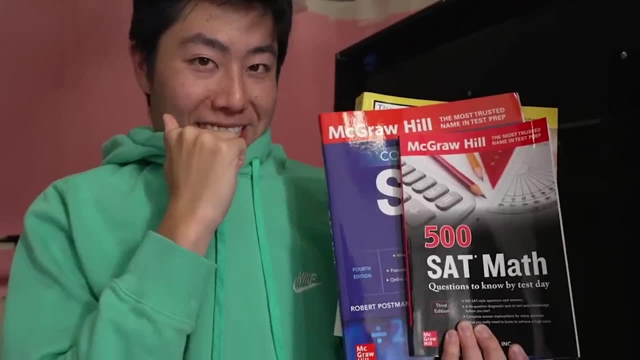 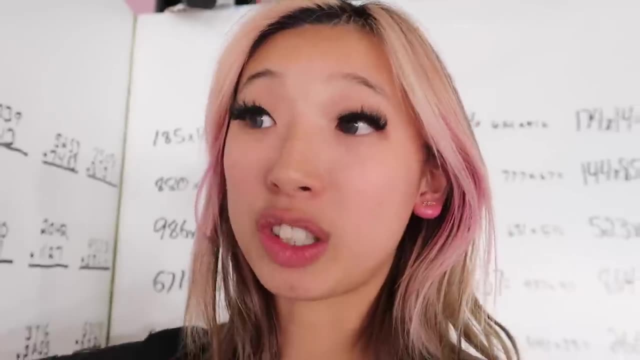 On her table she has a lot of workbooks. This was my nightmare back in high school. I did really bad on it, so don't ask me about my score. If you really think about it, I won't be able to keep up this pace for the whole 20 hours. 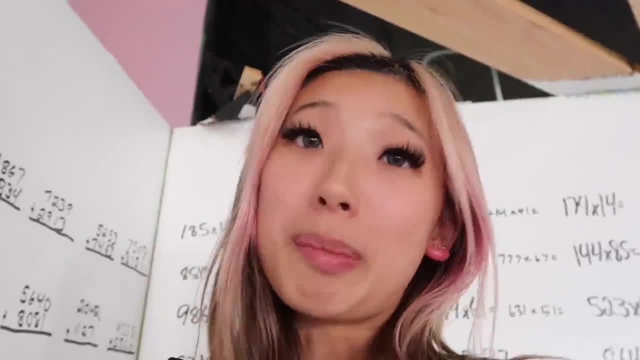 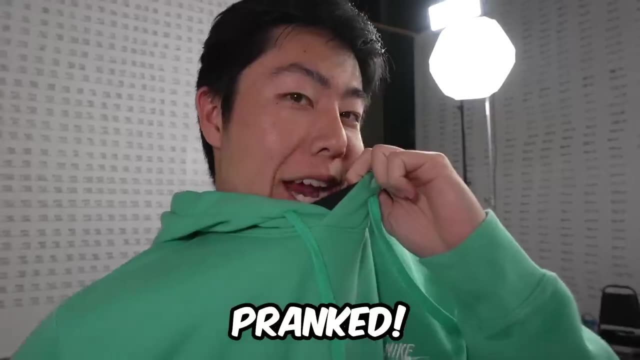 I'm gonna get sleepy. I'm gonna need to take breaks. I haven't even been to the bathroom yet. You're doing well, Michelle, Keep it up. Thank you, You're almost done with that wall Breaked. Two more problems left on this wall. 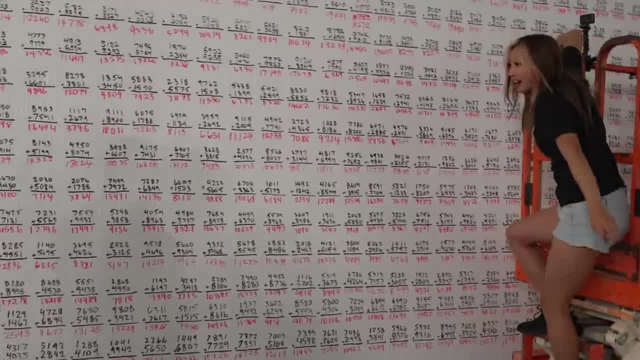 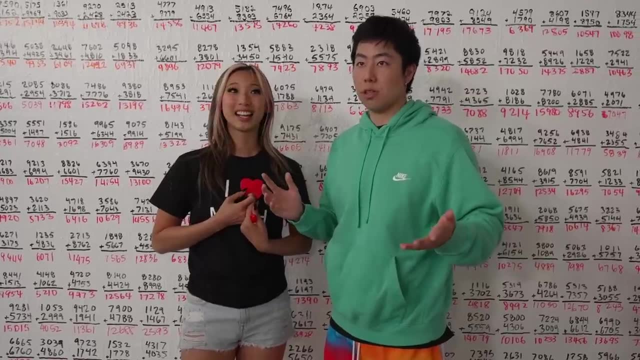 Yay, I am done with this wall. One wall done. Nice, I think I'm gonna eat. next, I can show you flashcards and you can say it: You kill two birds with one stone, but you don't want to actually kill the birds because 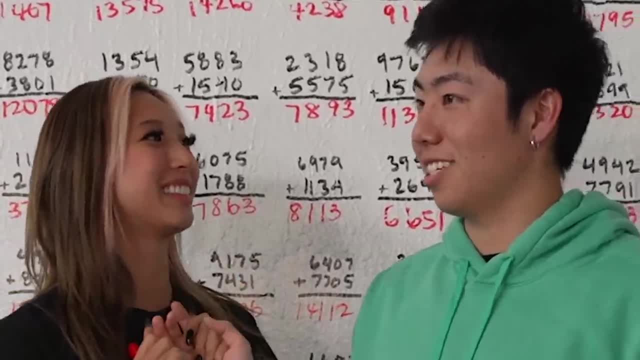 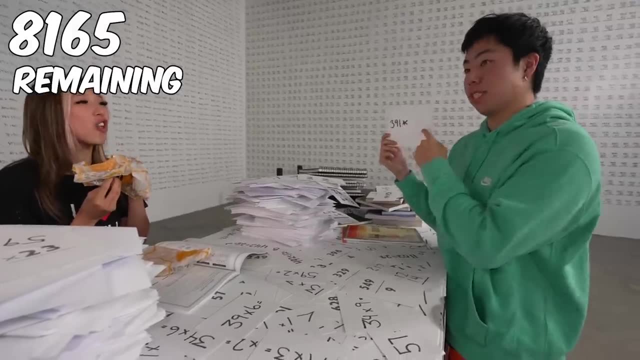 that's kind of mean. I have a plan: You hold the flashcards while I eat. Wait, that was my plan. 88, 144,, 136.. There's no math. Wait, I can do this 391 times. nothing, aka zero. 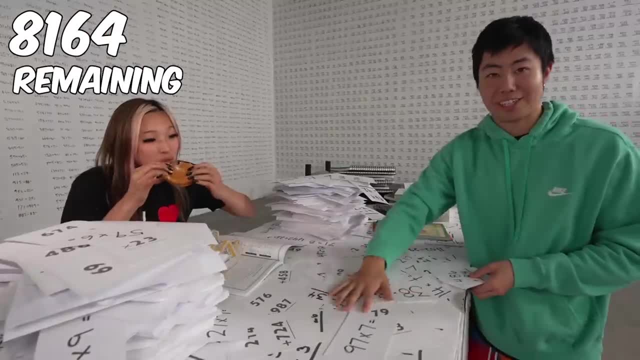 Zero, Zach, I need to go to the bathroom. Do you want to come with me? I need to collect a lot. This may take a while. Michelle's a psychopath. She's gonna eat while pooping. I'm hungry. 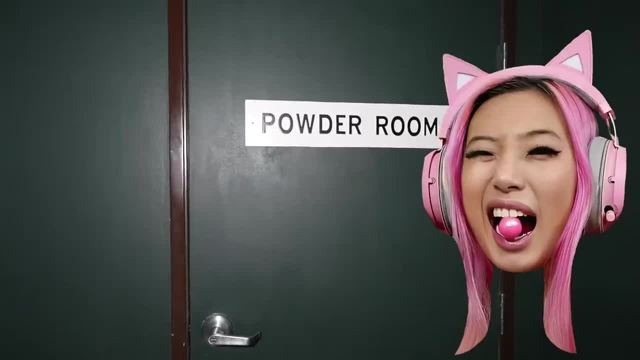 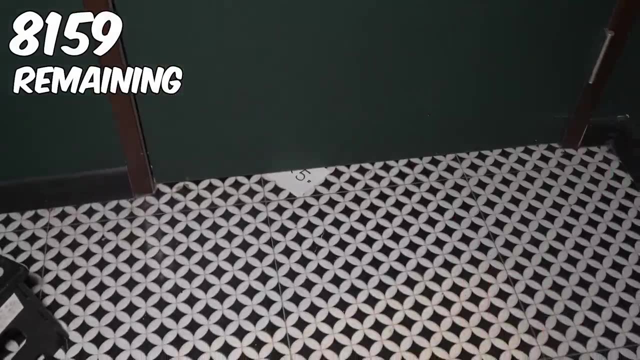 Ew, Stay there, Oh, Michelle. Oh, now I am 3-0.. How are you still eating? 1-975,, 223,, 204,, 169.. Zachary, don't open the door. Don't open the door. 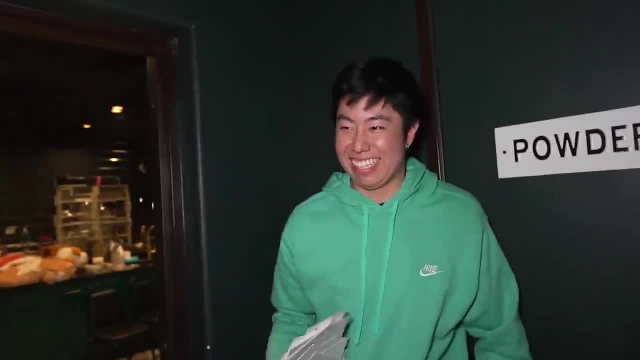 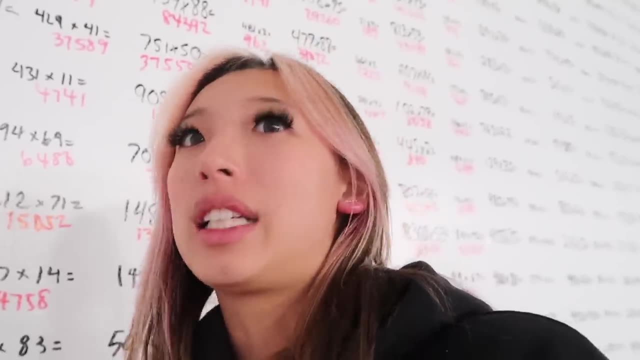 Zachary, don't open the door. My strategy right now is to finish the top row and then, when it gets later on at night and I get really, really tired, I'm gonna do more of the bottom without using the scissor lift. 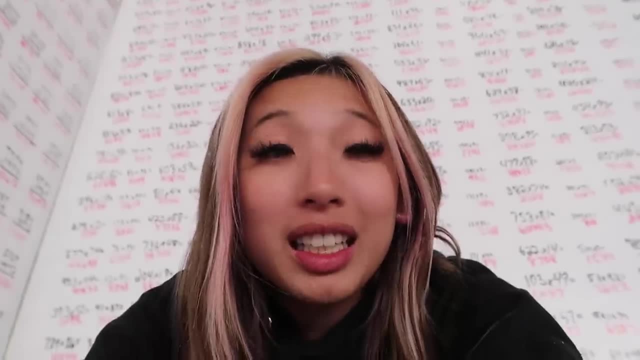 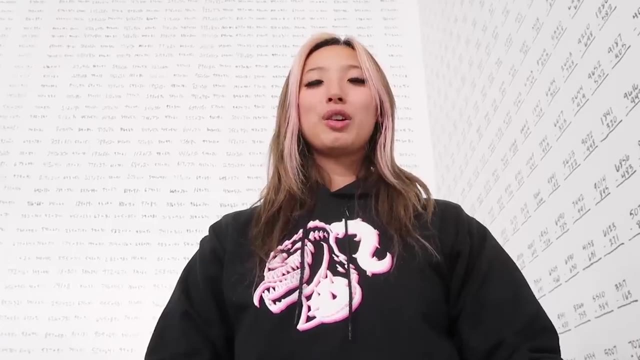 Look at how many multiplication problems I did. I know I should keep going, but I don't think I have the brain power to do that. Let's just meditate together, Breathe in, Breathe out. I'm really tired. 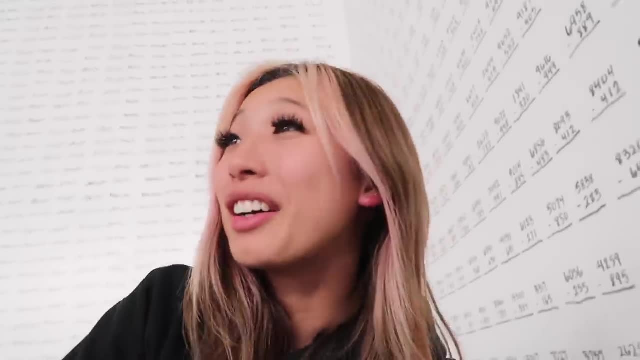 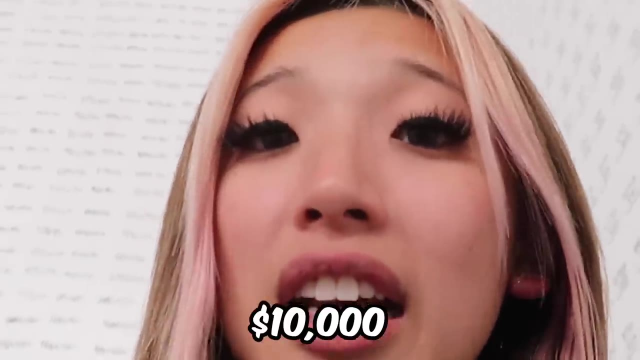 This is not the time to break down. I need to think about how I don't want the blue hair. And you know what, Michelle? If you keep going, I will be able to donate $10,000 to charity. Time lapse: 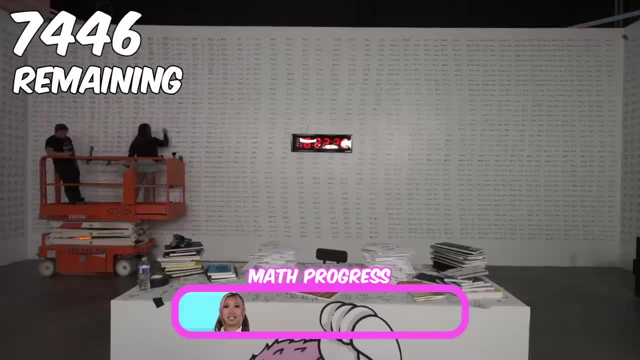 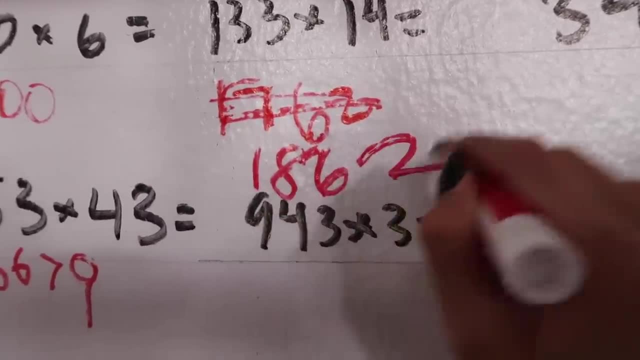 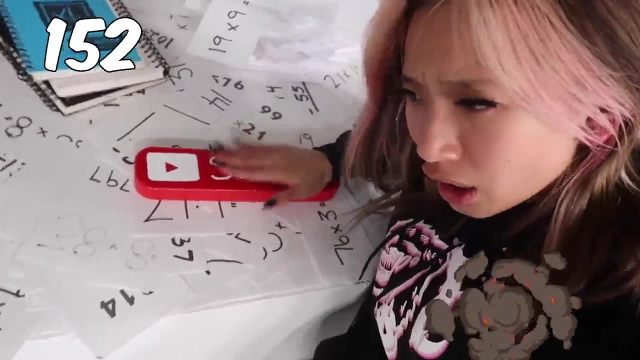 I got another problem wrong. It's 1-8-6-2.. Here's the subscribe button And I'm just supposed to press it 1,000 times. I can press really fast. You guys should press the subscribe button the way I'm pressing the subscribe button. 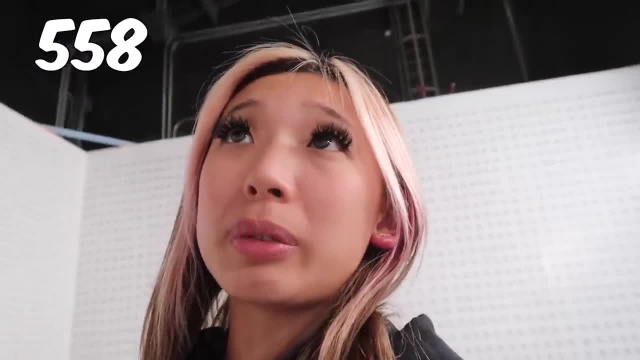 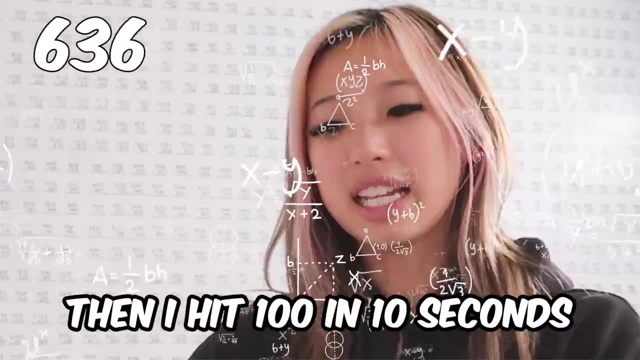 Smash it. If you do it 1,000 times, that means you subscribe, unsubscribe, subscribe, unsubscribe, So you should hit it 1,001 times. If I hit 10 in 1 second, then I hit 110 seconds, 100 in 100 seconds. 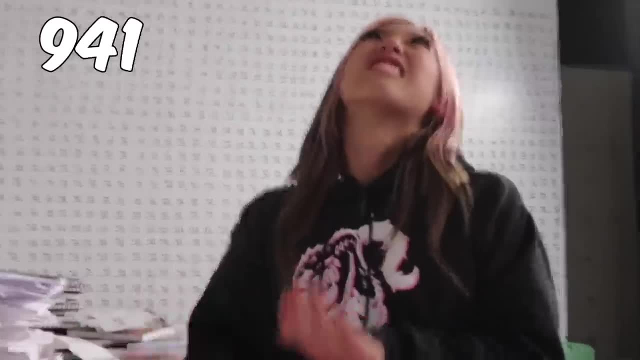 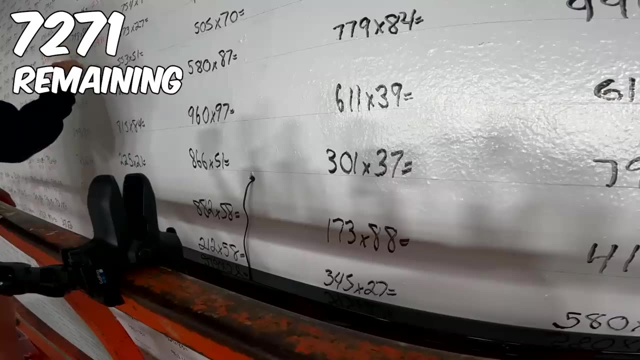 So I just need to hit this for 1 minute and 40 seconds- Done: This whole side of multiplication is done. I just have this side left. When I first walked into this, I wasn't thinking it was going to be hard. 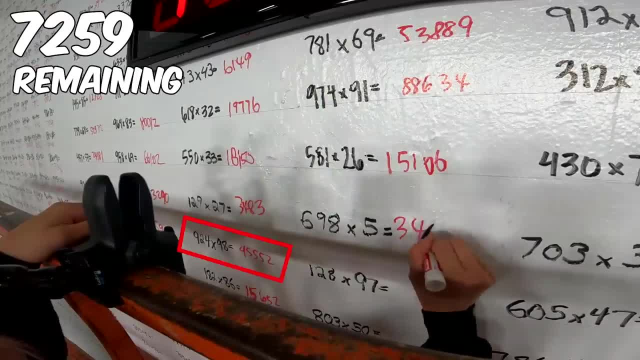 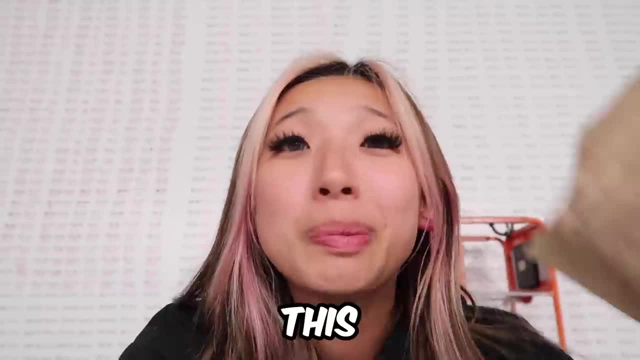 But the more I'm doing it, the harder it becomes. I got another one wrong. I don't know what's happening. I have to finish a bag of popcorn. This popcorn was popcorn Popped six hours ago, So soggy. 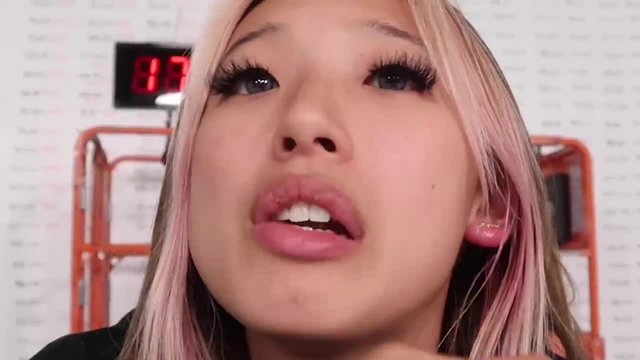 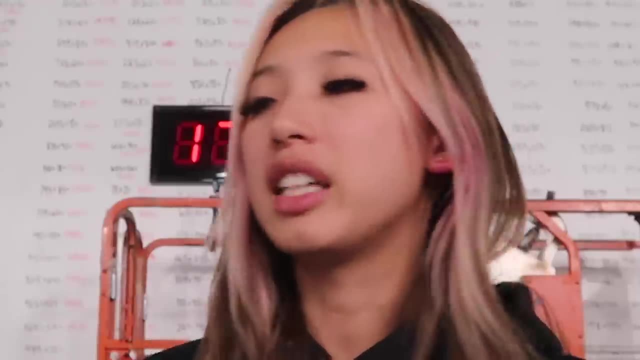 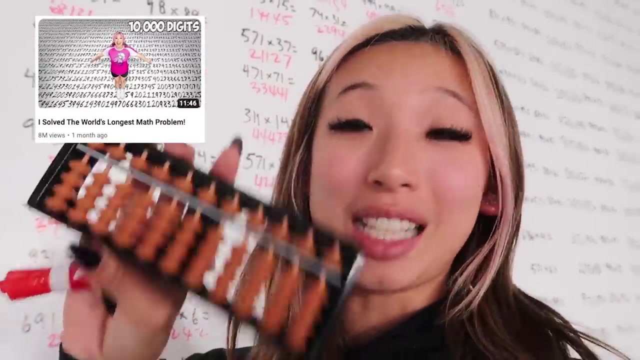 I have done math like this literally my whole life And never would I have thought that people would find it a little bit interesting. But I appreciate it a lot. Last one, Disgusting. In the previous video I showed you guys how to use an abacus. 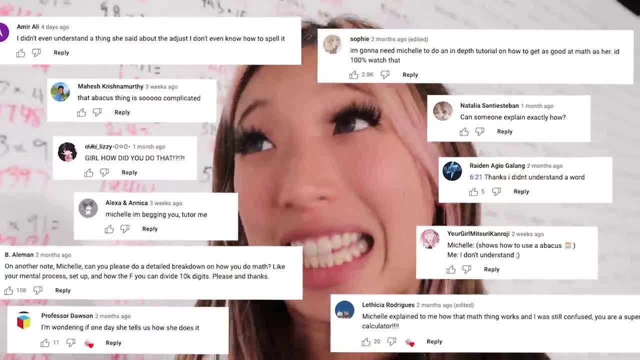 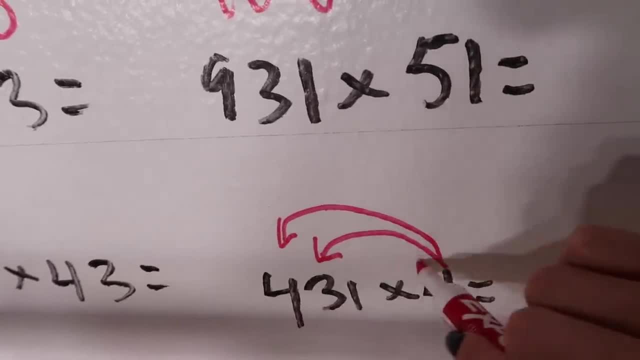 I've gotten a lot of comments saying that you guys didn't understand, So I'm going to try my best to explain it a little bit better. For abacus, you start from 4 x 4, then 4 x 3,, then 4 x 1.. 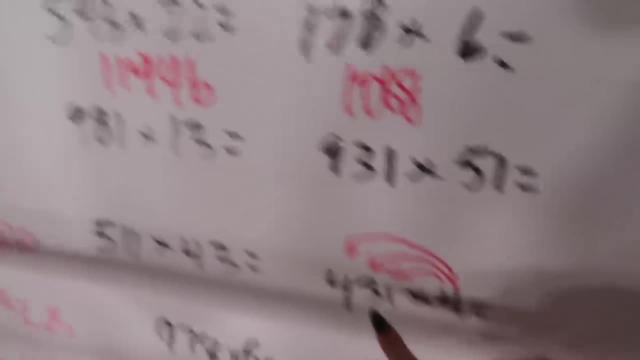 This is the 1 digit: 10, 100,, 1000.. This is a 4 digit answer, So we start on the 4th digit. So 1, 1,, 2,, 3,, 4.. 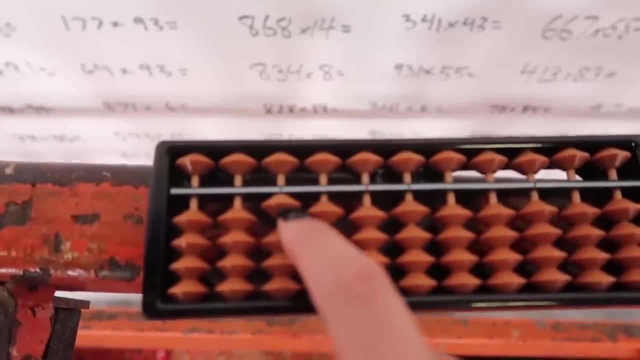 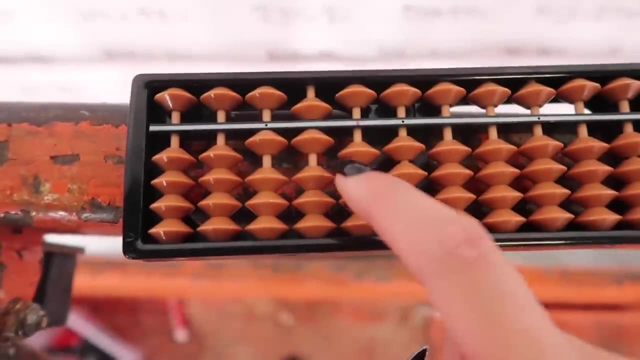 We start with 4 x 4, 16, 1, 6,, 1600 on the abacus, 4 x 3,, which is 12. So you add a 1 and then you add a 2.. 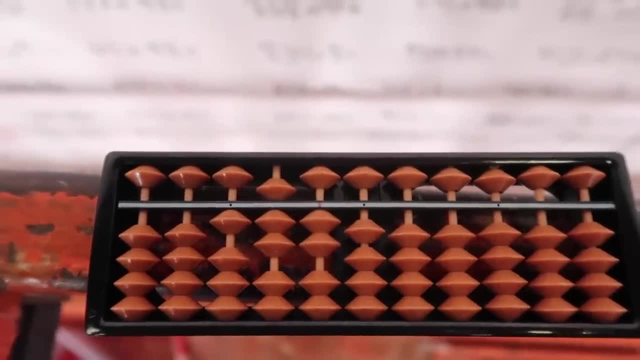 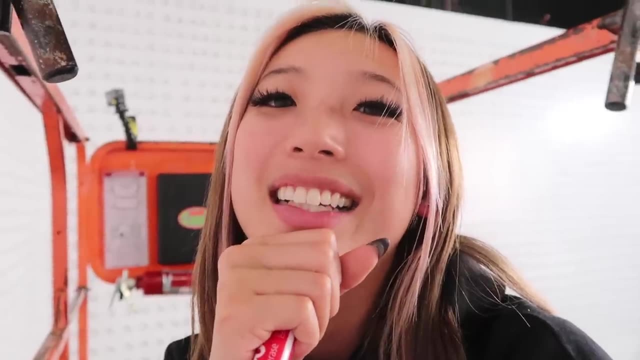 So now, so far on the abacus, I have 1,720.. So you do 4 x 1, you add a 4. And the answer is 1,724.. Let me know if you want another Miss Munchie abacus lesson. 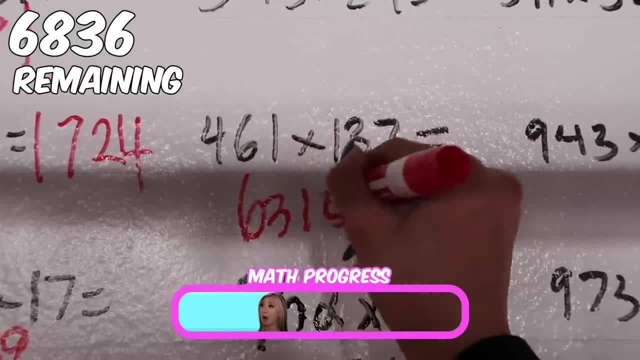 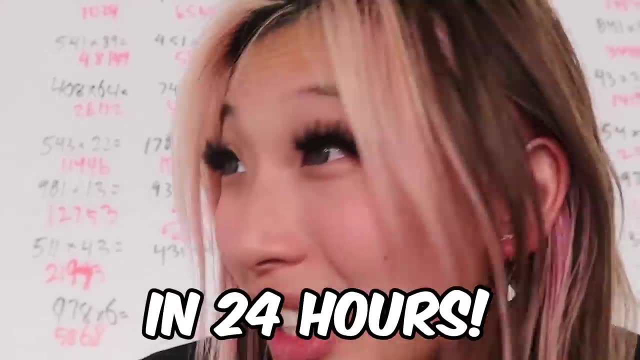 I'm getting really sleepy. Eight hours down, close to 3,200.. At this rate I will not be making it to 10,000 math problems in 24 hours. Blue hair can't be that bad. All of my other camera batteries I don't have. 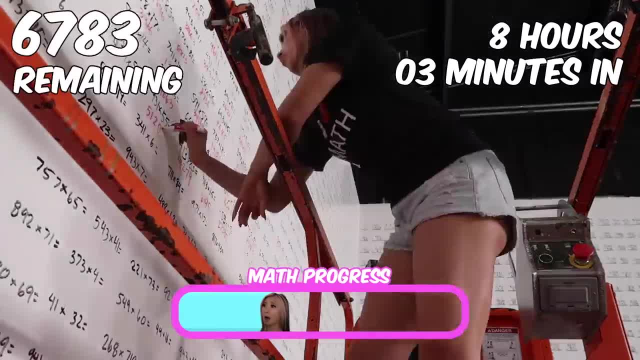 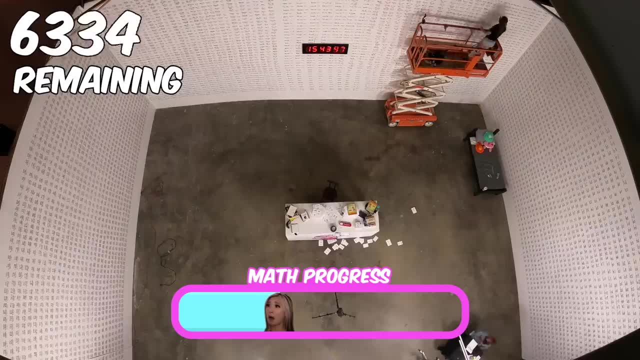 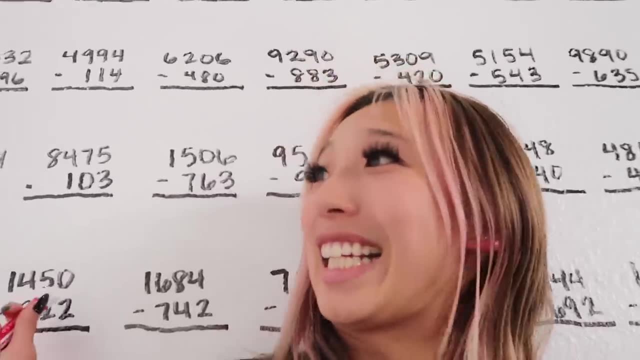 So please enjoy this awful time lapse. I've done all of the upper rows. Now all I have to do is zoom by the lower ones. I'm feeling very accomplished right now, But the bed looks so comfy I'm very dreading the subtraction balls. 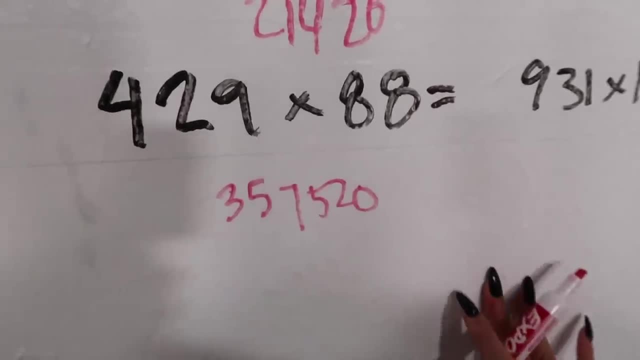 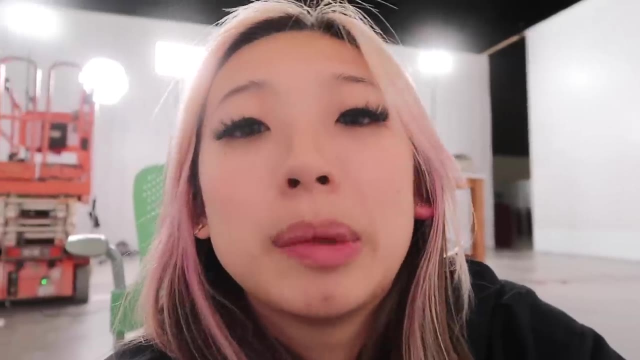 A 5 digit answer suddenly became a 6 digit answer And somehow 72 ends in a zero. I just I don't. This is the right answer. The next punishment on the list is an exercise die. Don't give me push-ups or burpees. 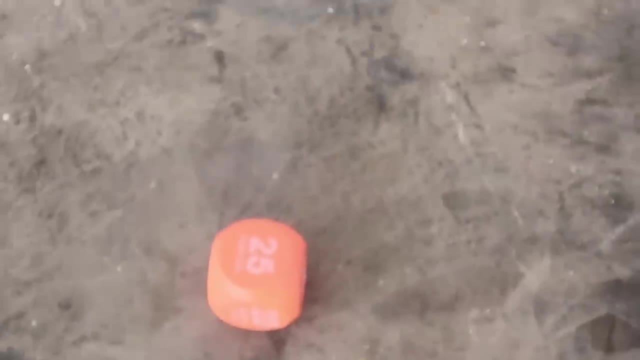 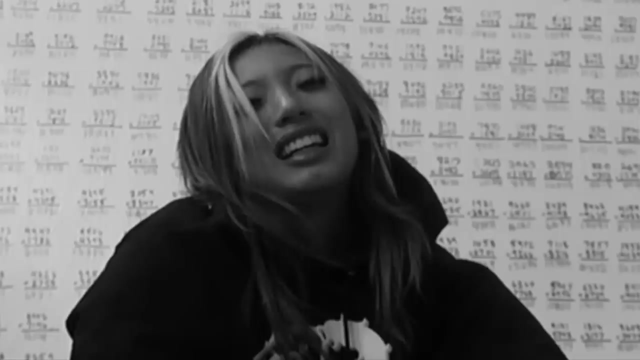 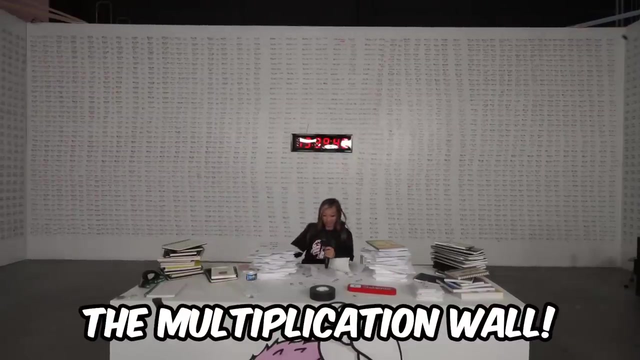 I don't feel like touching the floor. All right, what is it? Let's see about the push-ups. I'm so weak. Yeah, really fine, I just finished the multiplication ball. For the next couple hundred problems, I'm going to have to go to the gym. 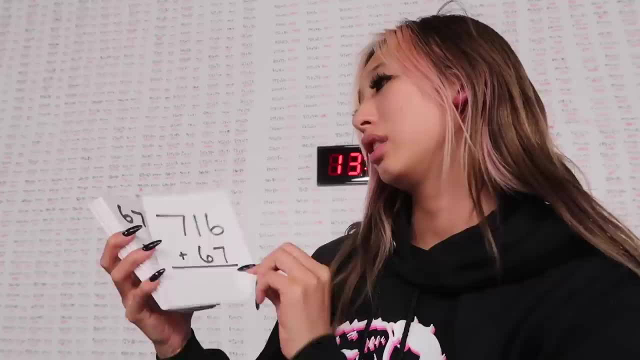 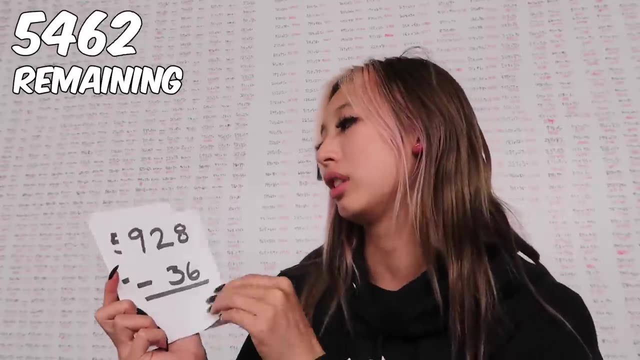 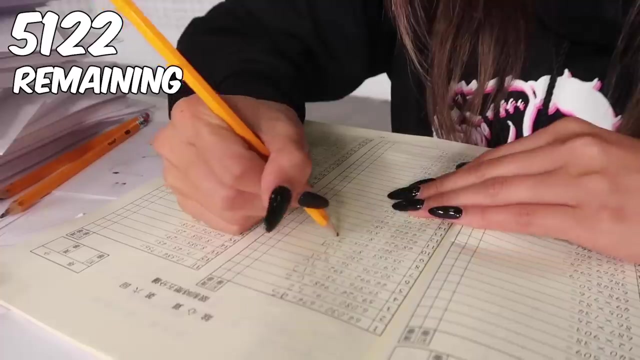 For the next couple hundred problems, I'm going to knock out these flashcards: 783,, 585, 488.. You can probably time lapse this 228.. 200 flashcards on the floor. I've officially hit 5,000 math problems. 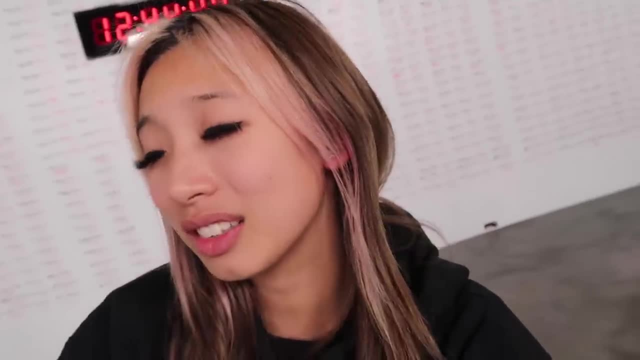 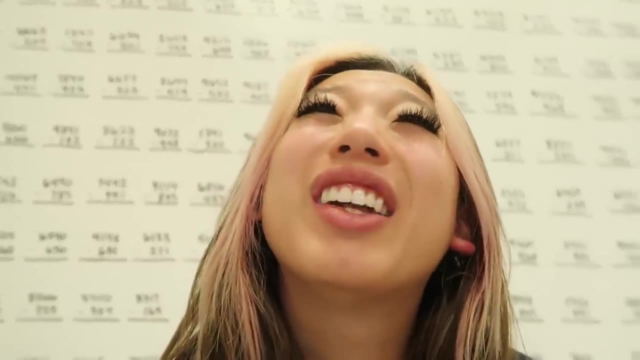 And I was able to do it in under 12 hours. I'm going to just take a quick, quick power nap. I promise I'll be right up. I wanted a 30-minute power nap but it turned into three hours. Let's get started on working on the subtraction wall. 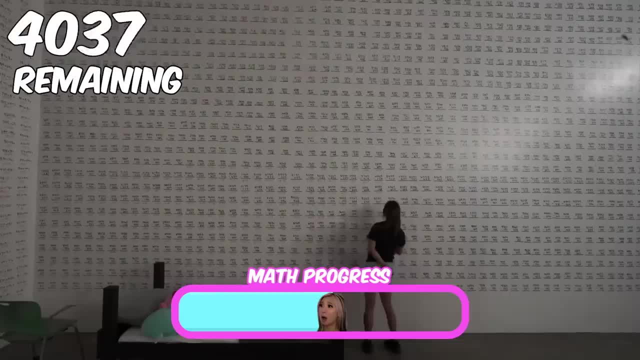 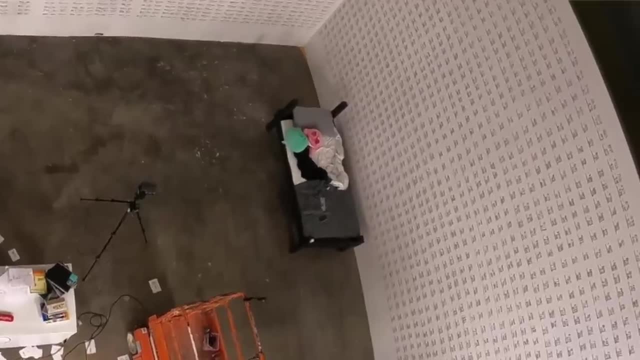 I ended up speeding through the third wall super, super fast. I'm almost halfway done with it. I'm on track to finish 10,000 math problems. As I'm writing these math problems, I was thinking about how my whole social media career. 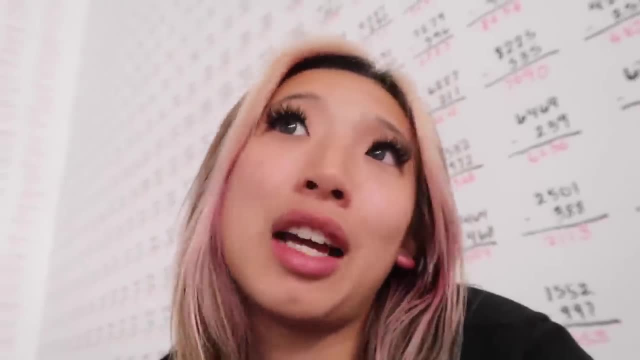 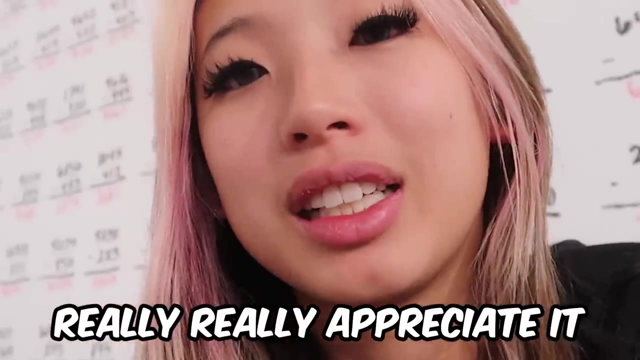 people wouldn't really care about me or watch me if Zach wasn't there. The fact that you guys are still watching this is so amazing, And I really really appreciate it a lot. I'm a little bored And I kind of wanted to call up Zach. 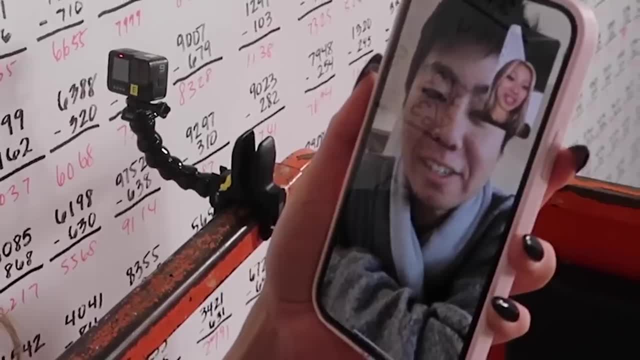 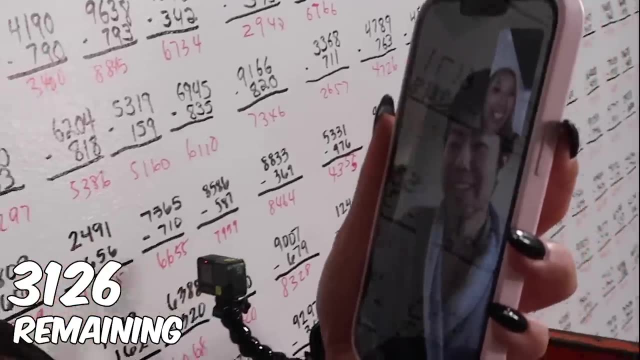 You're awake. Guess what? What? I'm naked underneath. It's okay. Anyway, I'm calling you because I'm bored, So give me a math question: 1 plus 5. 6. Plus 1. 7.. 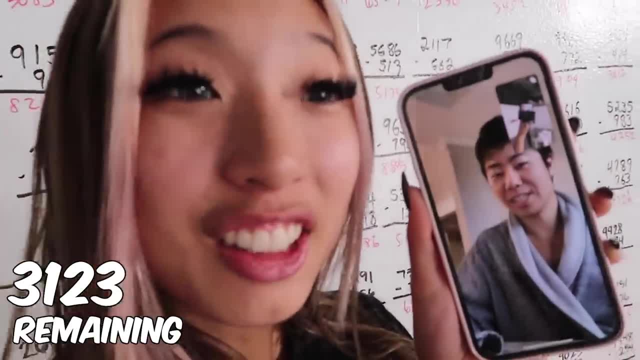 Plus 1., 8. Plus, 2., 10. Plus, 3. 13. Plus, 4., 14., No 17,, 17,, 17,, 17.. Wait, these are easy, Michelle, You just got one. 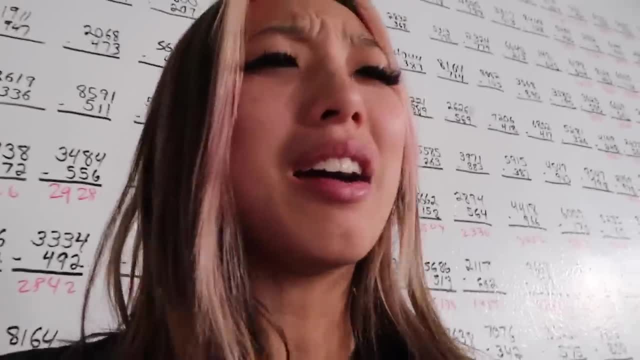 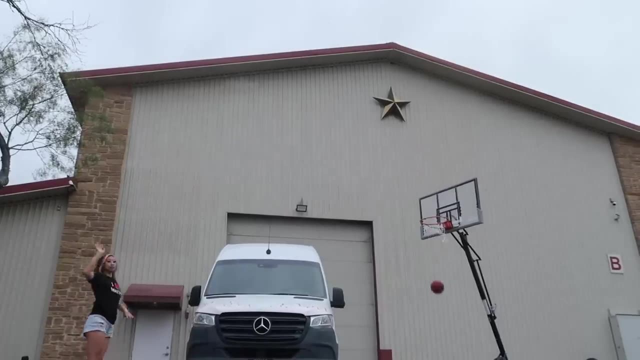 What's wrong? You messed me up. Oh, I like basketball, So you need to make a three-pointer like Curry, Easy Curry. All right, let's call up my friend Isaiah. All right, give them to me 4 times 4.. 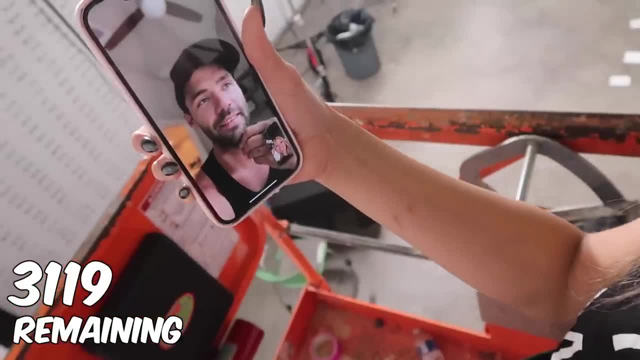 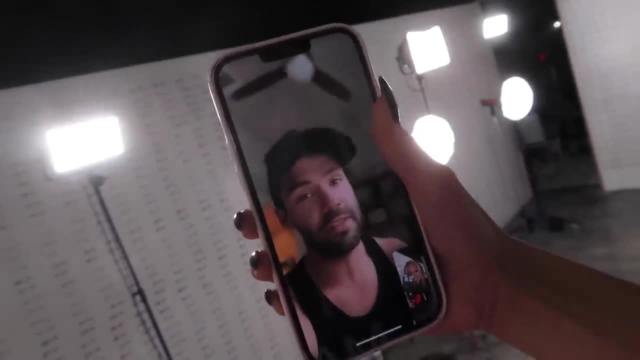 16. 16 times 16. 256.. 256 divided by 2. 128. 128.. OK, You just have to stay focused and remember that it's too easy. OK, I'm going to call up Zach's mom. 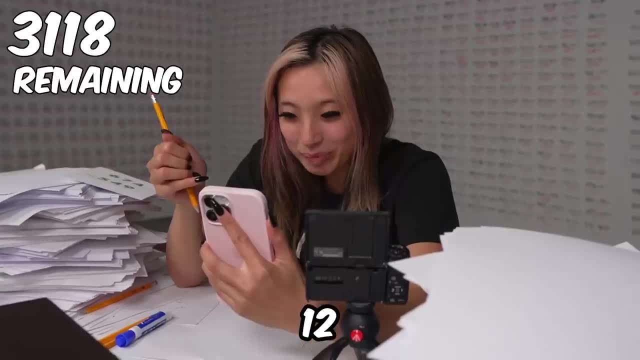 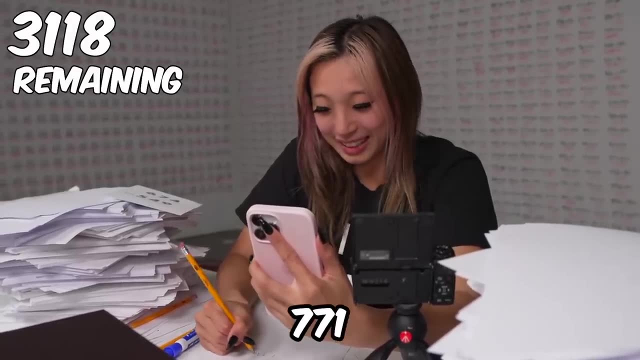 All right, I was wondering if you can give me some math problems: 1, 2,, 3,, 4,, 5, 6 divided by 16.. OK, 7, 7,, 1, 6.. 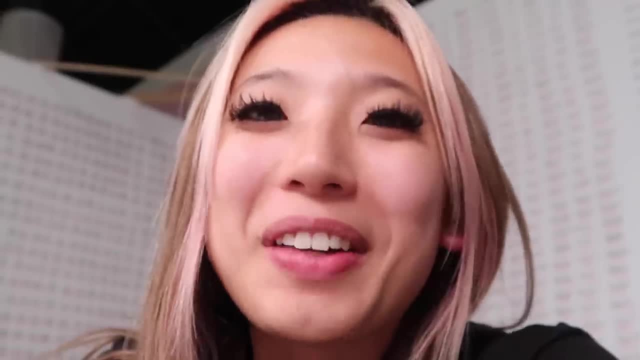 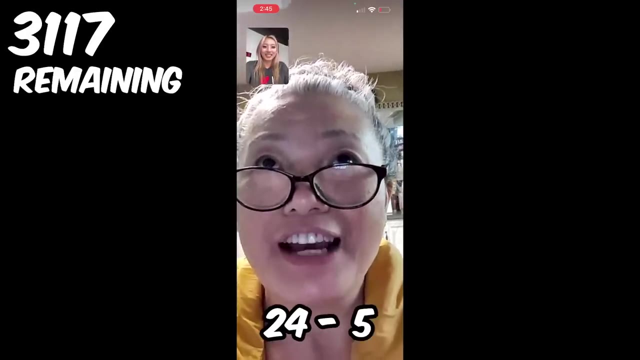 Thank you, No problem, Good luck Next up. I'm going to call my mom. Hi mama, Do you think you could give me some math problems? 24 minus 5 times 24 plus 100 divided by 24.. 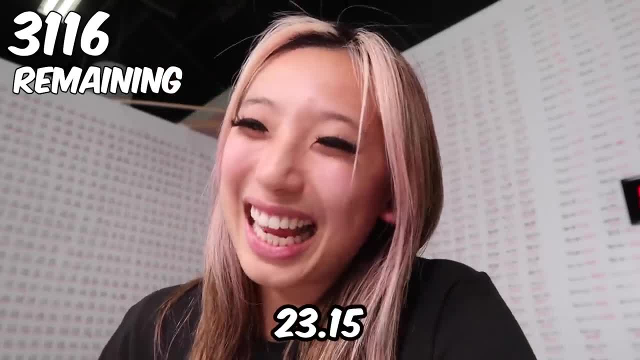 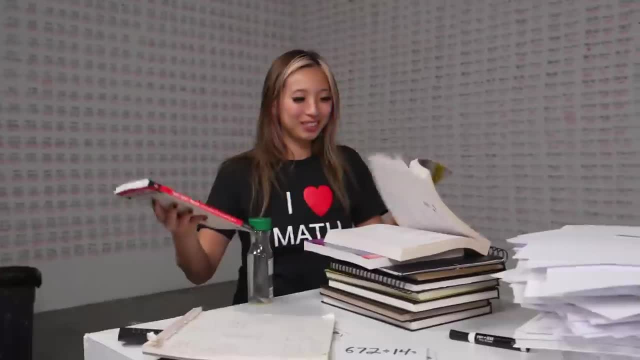 Mama, that's a lot: 23.15.. 23.15 is the answer. You're faster than a calculator. Oh, thank you, mama. And workbook time- Oh my gosh. I feel like I can do a couple of these. 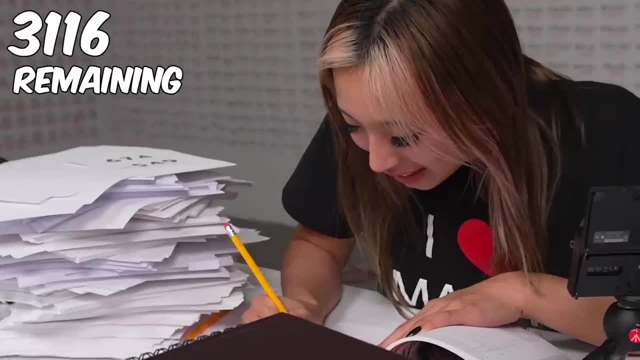 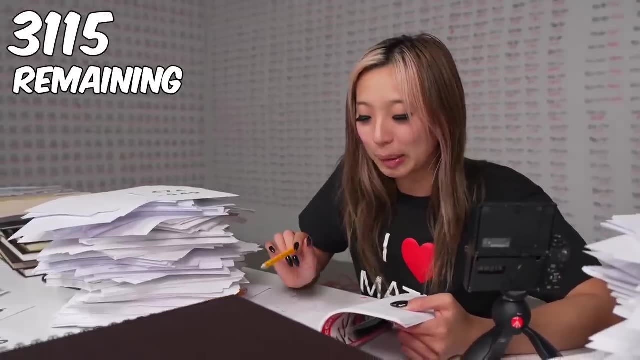 2x plus 4 equals 4x minus 2.. 6x equals to 3.. x is 17.. This is going to take forever. a, b, c and d are all different numbers of different values, So it's a plus 3 equals a- b. 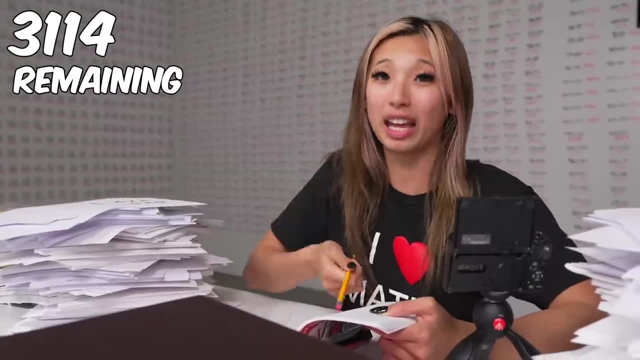 So a times 3 times 3 equals a 0.. Huh C Easy. Because if a or b is 0, then that means a plus 3 equals a b. Because if a or b is 0, then that means a plus 3 equals a b. So if a or b is 0,, then that means a plus 3 equals a b. So if a or b is 0,, then that means a plus 3 equals a b. So if a or b is 0,, then that means a equals a b. 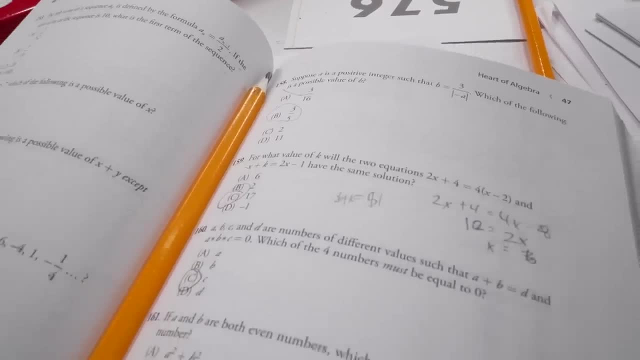 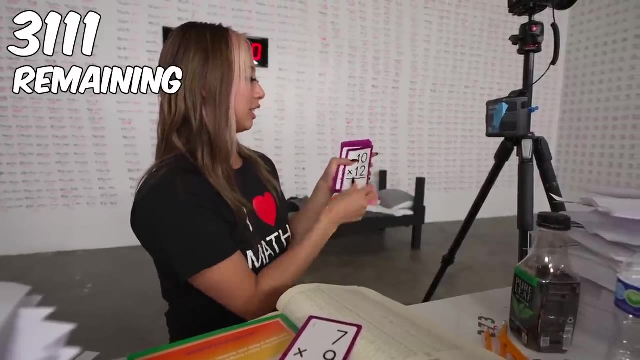 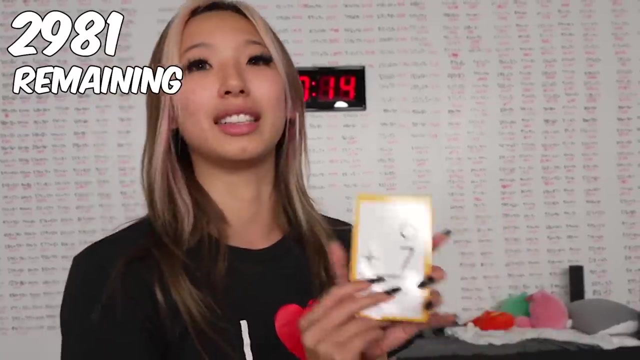 Or b equals a b. if that can't be true, This proves that I can do more than just arithmetic. I can do ACT math: 44,, 66,, 64,, 16.. 1,, 2,, 3,, 4,, 10,, 11,, 13,, 14,, 11,, 13,, 8,, 12,, 13.. 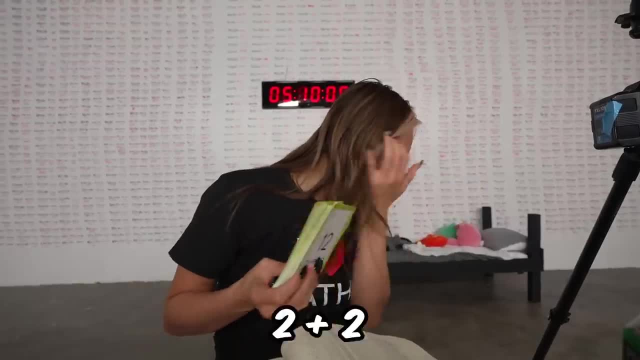 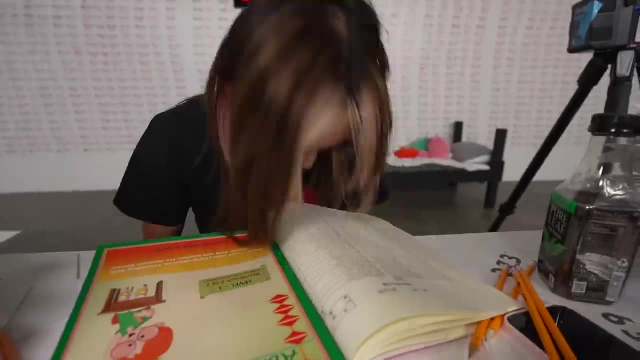 I hate to do this, but you got one wrong. Oh which one? 2 plus 2, you said 14.. I said 14. 14. 14. What's my problem? I'm listening to a stupid alarm for five minutes. 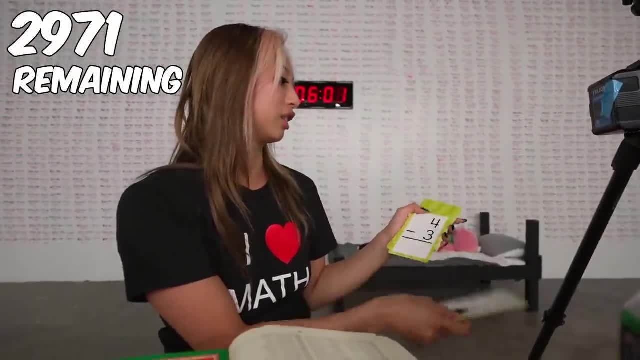 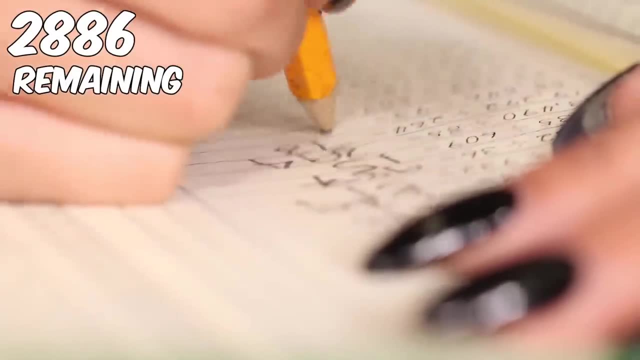 2, 1, 0, 4, 3, 2, 1.. That's what they teach you in human calculator school. They actually play alarms like that, And I have to do math problems. That's enough. 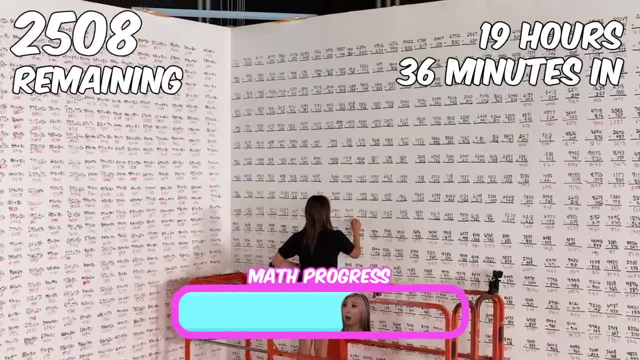 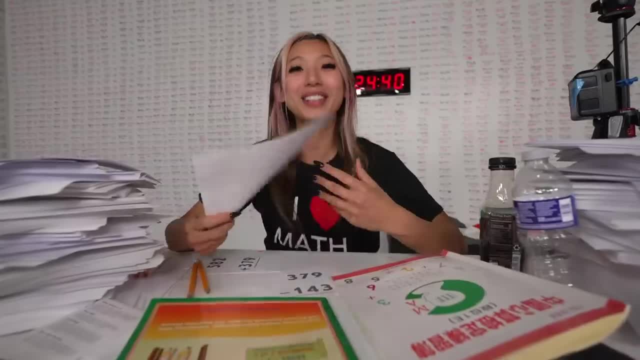 That's enough Before I do the division wall. there's a bunch of lights over there that the videographers have to move. While I wait for this, I'm going to work on these worksheets: 3,, 2,, 1, go. 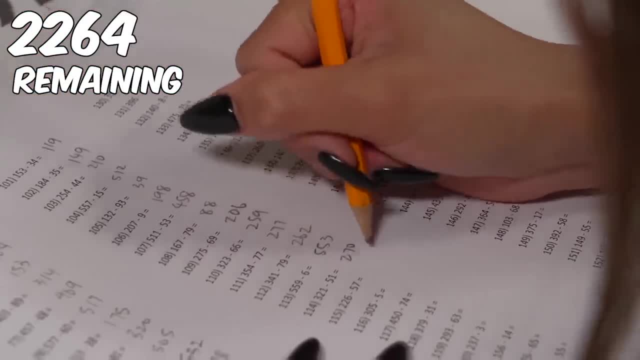 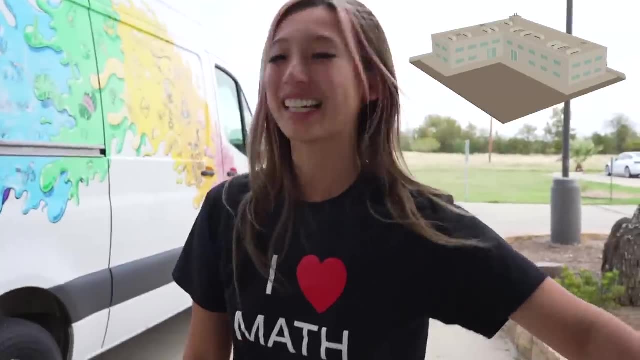 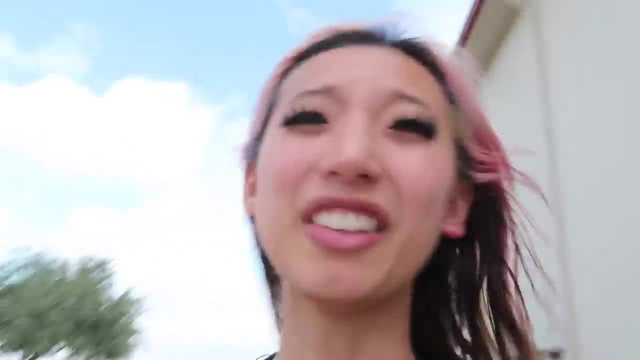 For every question I get wrong, I will run the lap around this building Teacher 17.. Boom, 17 laps. I'll be right back, guys. I wasn't expecting to get this many wrong, So I don't know if I'm going to finish in time. 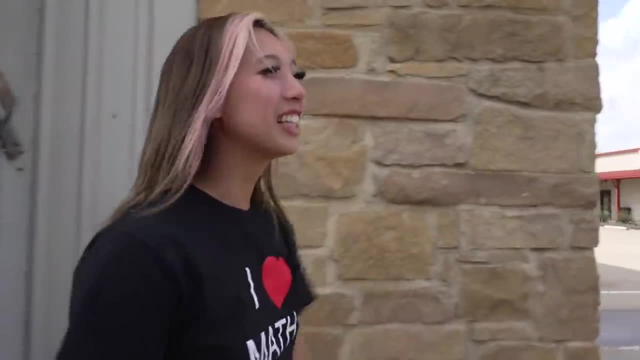 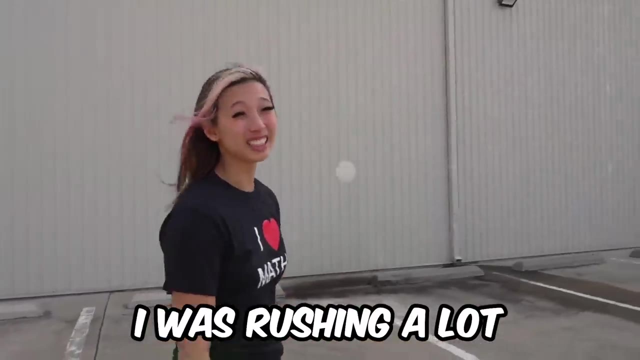 I'm a little bit worried. I can't believe I got 17 wrong, But throughout the whole wall I didn't get anything wrong. I knew I got a lot wrong in the end because I was rushing a lot. Learn from me. 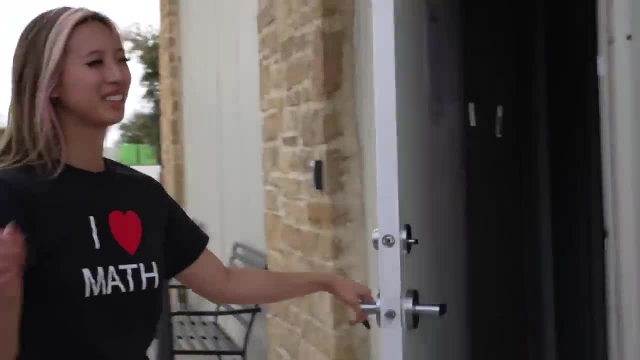 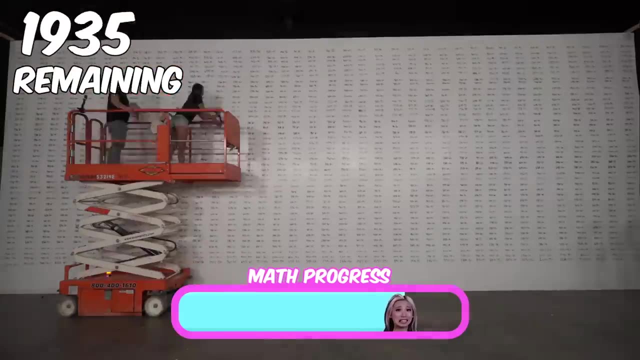 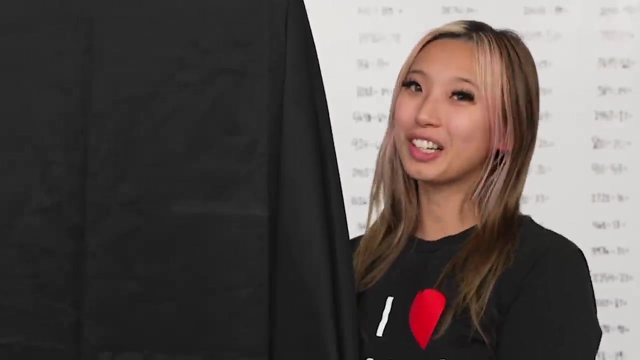 I'll waste off a decade. Let's go back to doing math. The vision wall is ready to be solved. I'm going through these so fast. I love the vision so much, So before I finish the last 1000 problems, I want to do a quick competition with you guys. 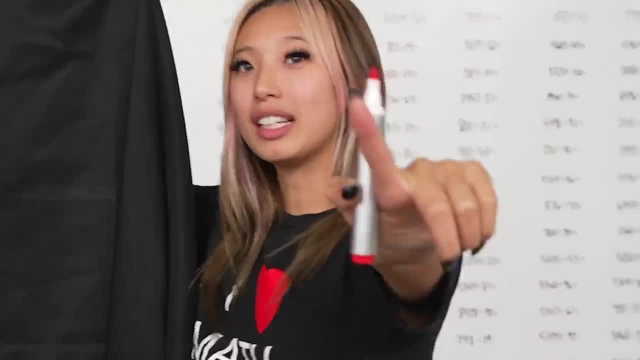 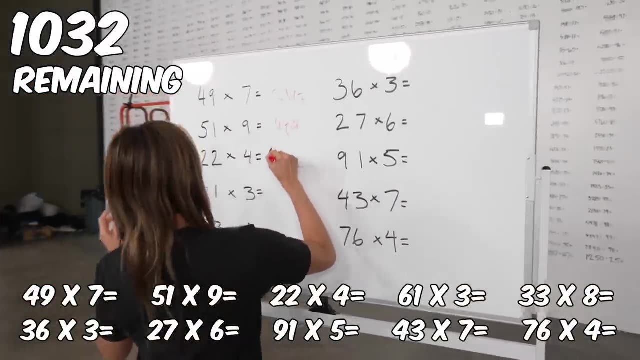 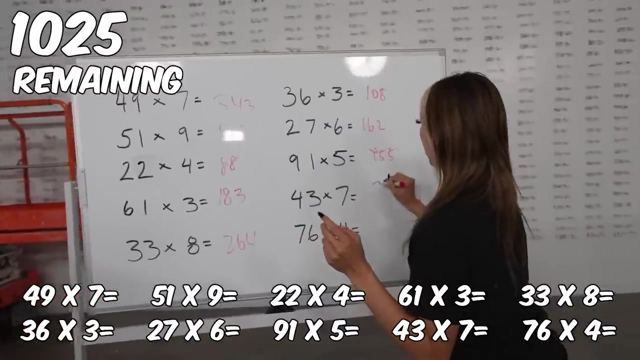 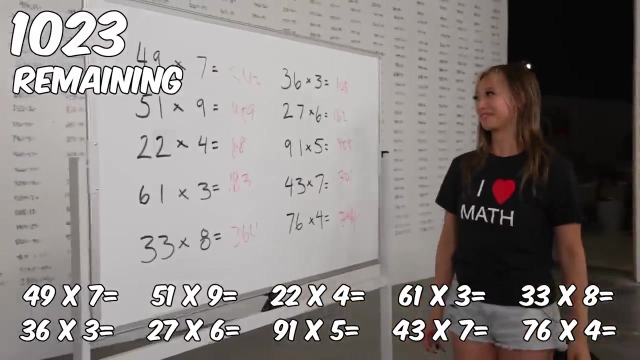 I've never seen the problems behind this whiteboard. Once I ink it off, the timer starts. Get your pens and paper. Paper is ready. Okay, ready, Go Done. Well, I was sweating after that. That was a tough competition.